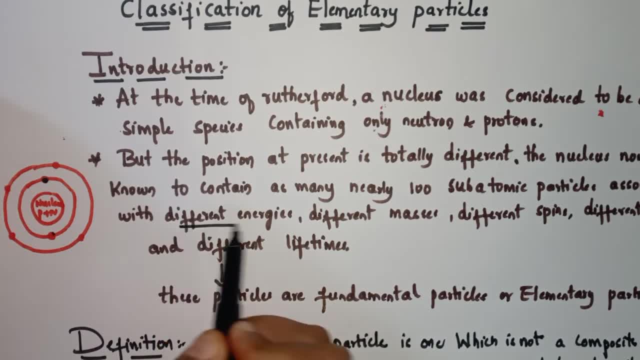 subatomic particles associated with different energies, different masses, different spins, different charges and different lifetimes. These are called as that is, these particles are called as fundamental particles or they are also called as elementary particles. Now let's see the definition of these elementary particles. 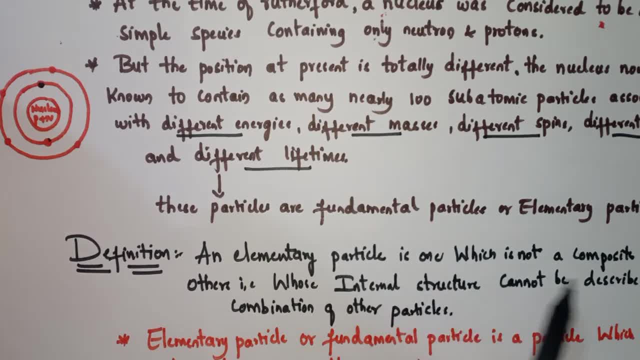 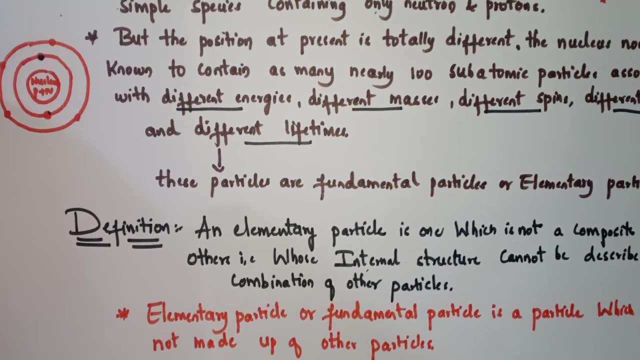 Here. an elementary particle is one which is not a composite of others, that is, whose internal structure cannot be described as a combination of other particles. In simple terms, we can say that elementary particles or fundamental particles is a particle which is not made up of other particles. 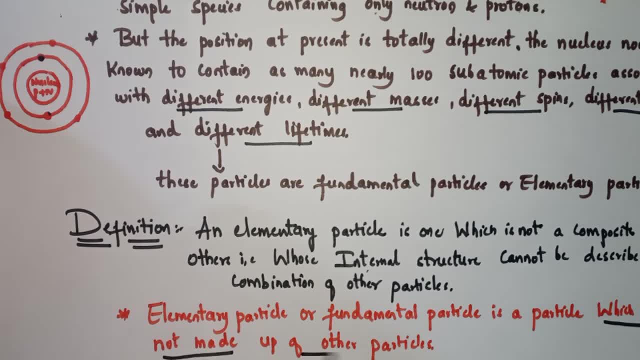 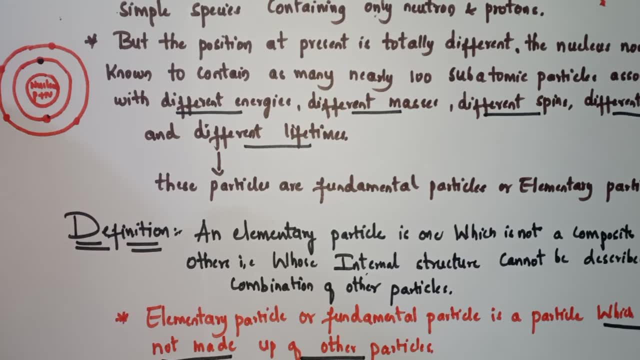 This is very, very important. that is, it is not made up of any other particles. There is no combination of other particles in these elementary particles. This is about the introduction and definition of these elementary particles. Now let's see the classification. Now let's see the classification of elementary particles on the basis of characteristic. 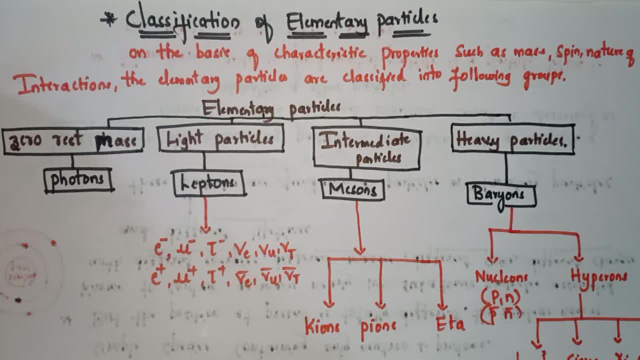 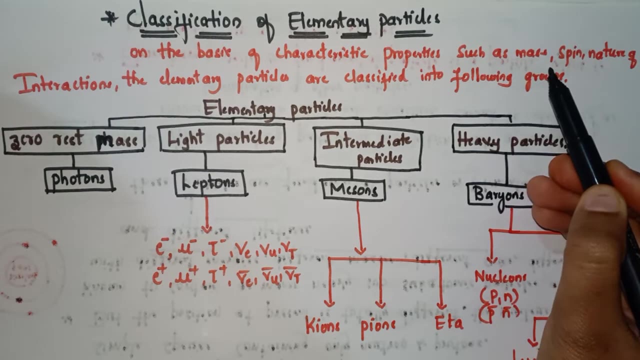 properties such as mass, spin, nature of interactions. So now, by the following basis, the elementary particles are classified into the following groups. See here the important thing, that is, on the basis of mass, the classification of elementary particle is different On the basis. 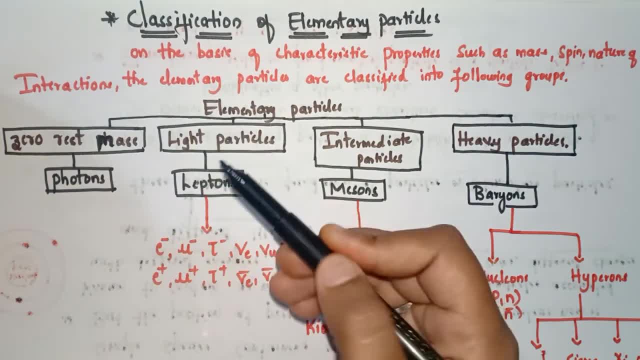 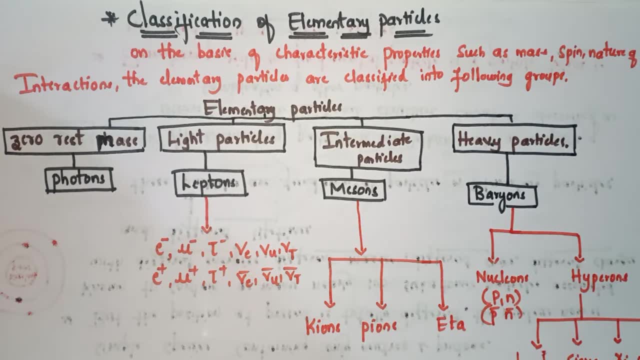 of spin it is different and on the basis of nature of interaction. also, classification of elementary particle is different. But I have combined all these things and I have done a flow chart to make you understand it better. So let's start with this classification Now. 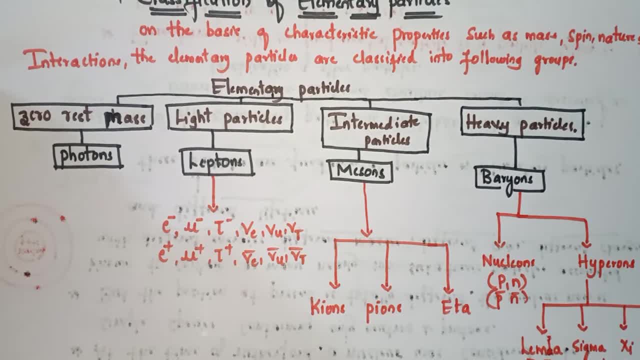 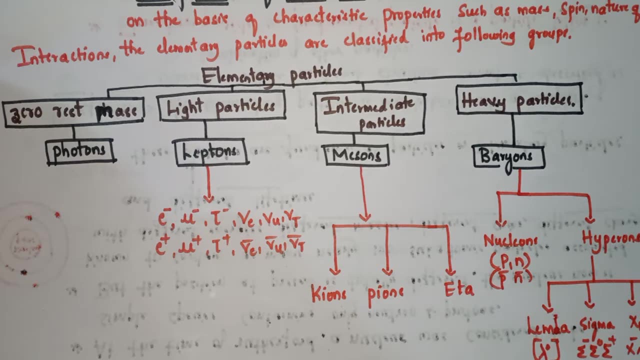 the elementary particles. as I have already told, it is classified on the basis of mass. Here an elementary particle, as always, has the same rest mass. Now, here, on the basis of spin, the particles of off integral spins are different and particles having zero or integral spins are: 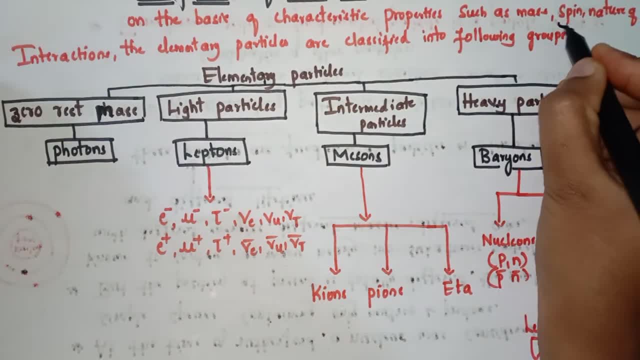 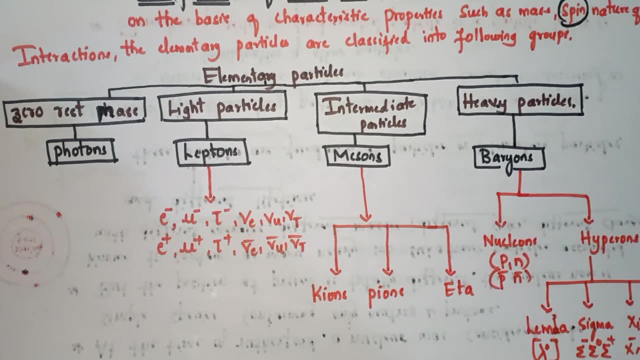 different. I will explain you it later. Remember this. spins. Now, coming to the nature of interactions. the interaction may be gravitational interactions, weak interactions, electromagnetic interaction or strong interaction. Based on the nature of interactions, the interaction may be much more complex than the natural interaction. Therefore, on these things, we have classified. 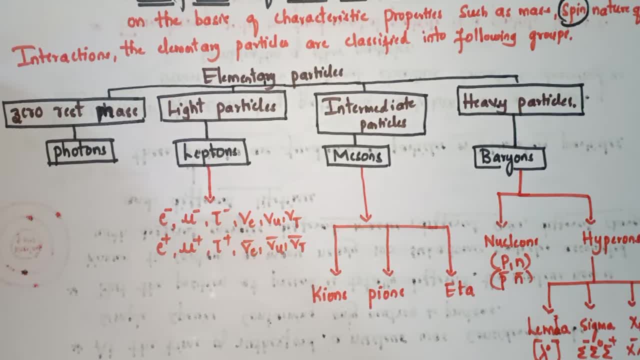 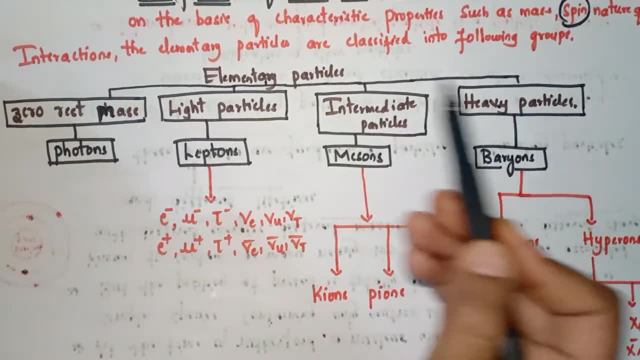 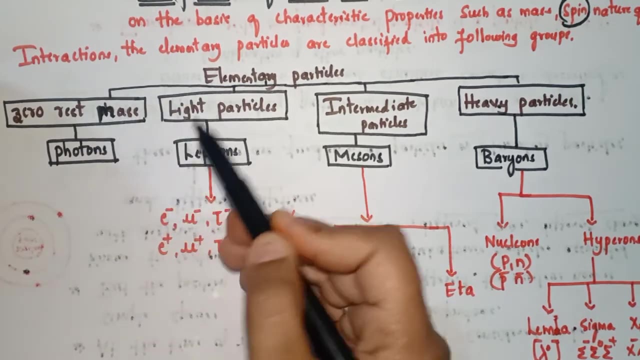 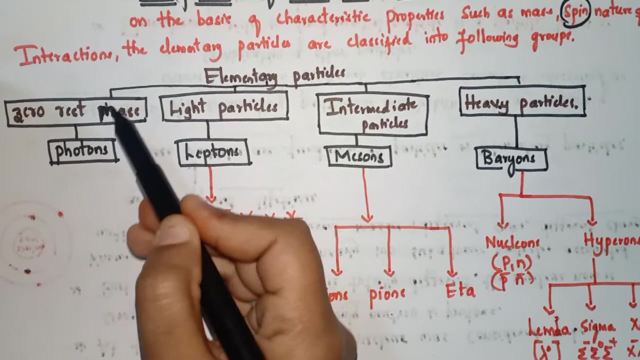 the elementary particles like this. Now let's understand this classification. Now elementary particles are classified into four types. First it is having zero rest mass, then comes light particles, then comes intermediate particles, then comes heavy particles. Under the zero rest mass particles we have protons For. 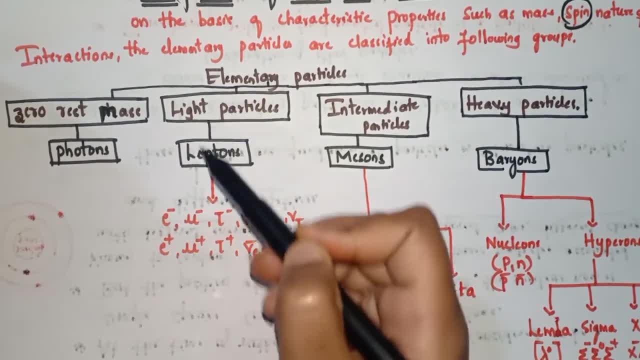 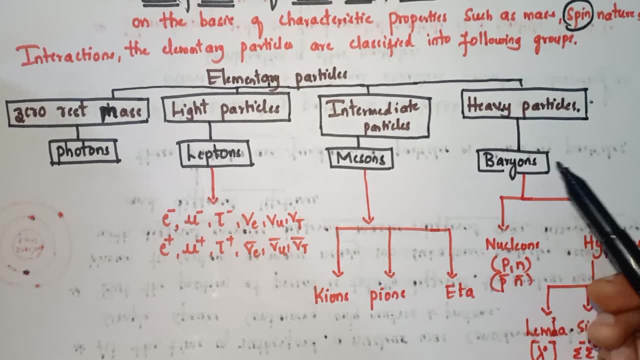 light particles we have protons, And for the light particles we have protons. For particles we have leptons, light particles, leptons, intermediate particles, mesons and heavy particles, baryons- here photons are not classified further here. and then, coming to the light particles, it 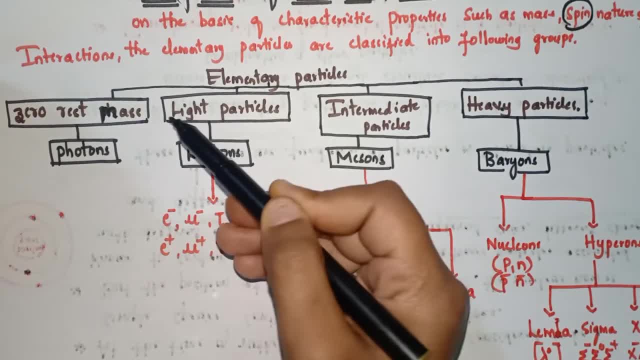 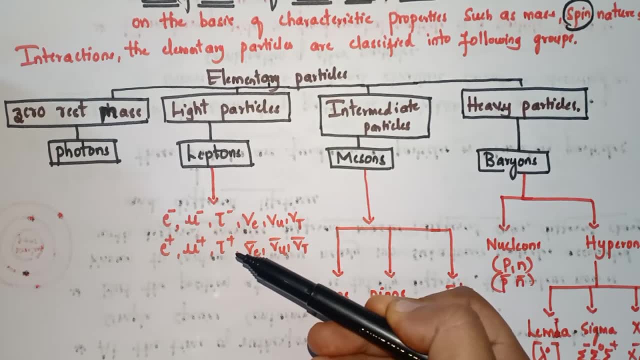 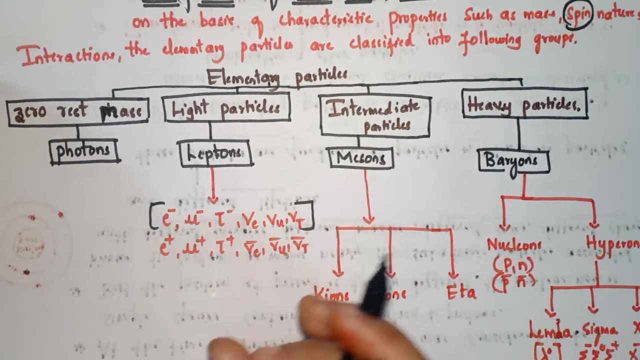 is classified into leptons. i have already said that, like that, light particles are classified into leptons, they are further classified into 12 types. just remember this: above these six, then you will come to know what are the other six here. see here leptons are classified into. 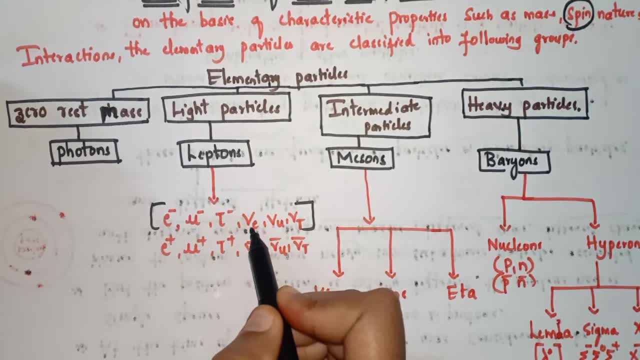 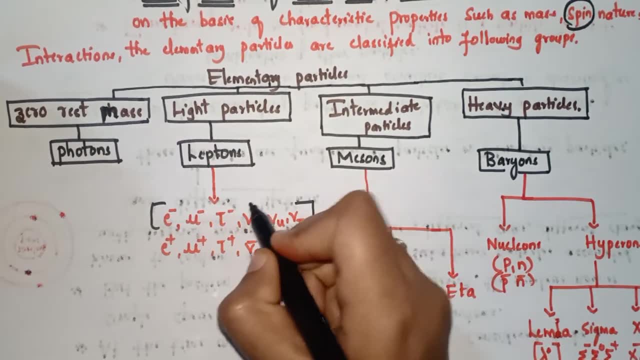 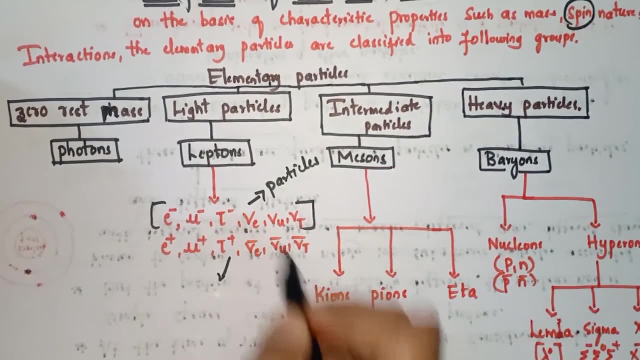 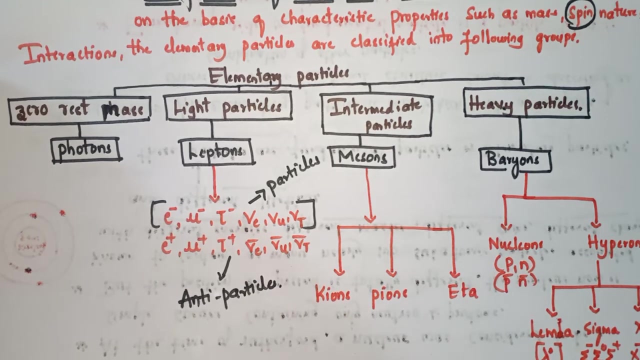 electrons: mu minus tau minus electron neutrino, mu neutrino and tau neutrino. these are the particles. now for these particles we have to write the anti-particles. the below things are anti-particles. now, direct, direct predicted theoretically that existence of anti-particles for the electron. 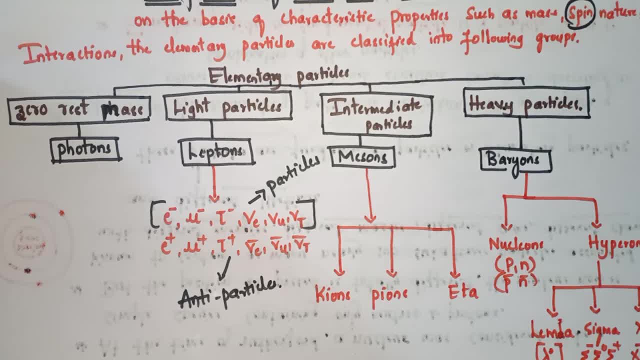 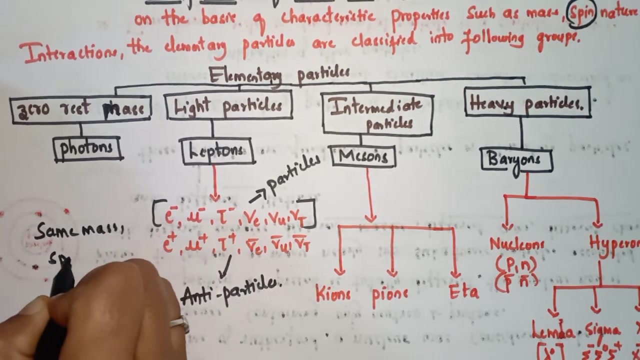 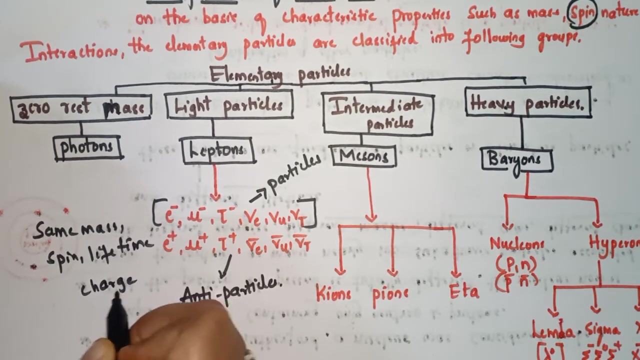 he actually postulated that every particle has a anti-particle. these upper things are particles and these below things are anti-particle. see see here anti-particles of a given particle as exactly the same mass, pin and lifetime. they are having same mass, spin, lifetime, but they are only differing in the charge. if it is having, the particle is having. 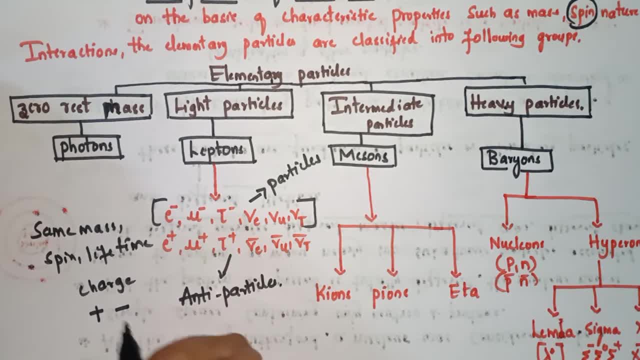 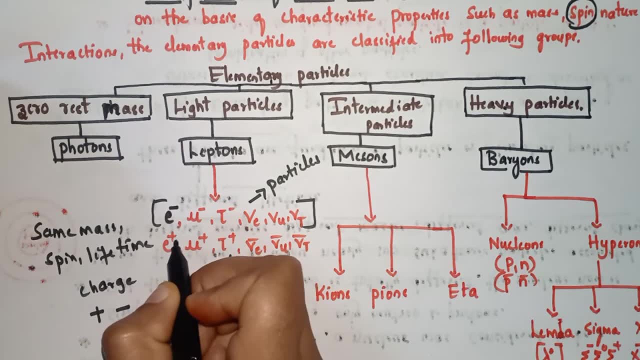 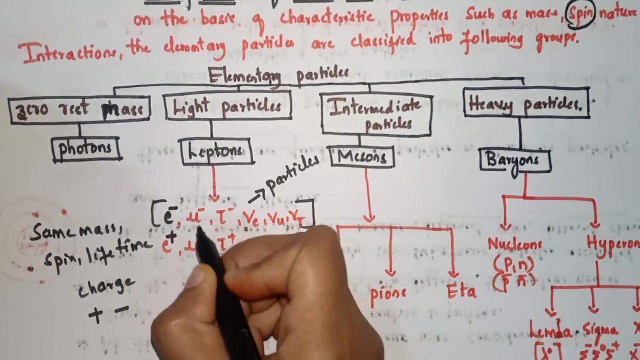 positive charge means anti-particle will have minus charge. that is negative charge. here it is the electron and further electron. if we have positive charge then it is called as positive- sorry, positron. so e minus is a particle and e dole plus is an anti-particle. 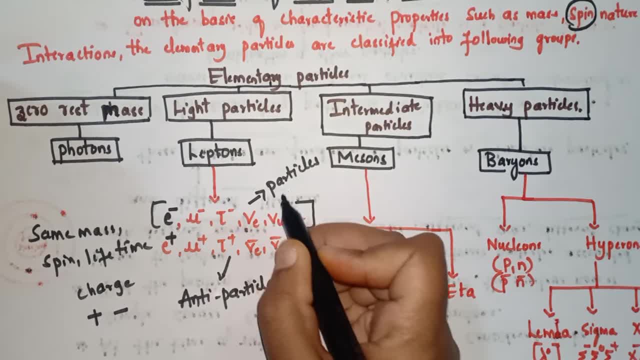 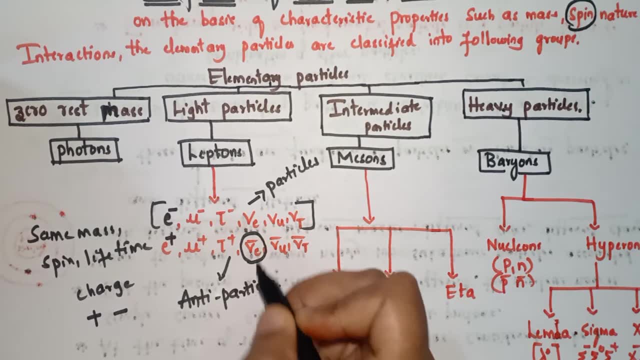 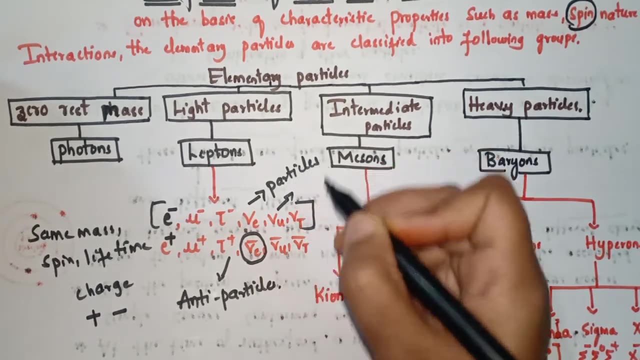 mu minus in the particle and mu plus is a anti-particle. tau plus is an anti-particle. electron neutrino is a particle and it is electron anti neutrino timeframe. it is a anti-particle. this is new neutrino. new neutrino is a particle. 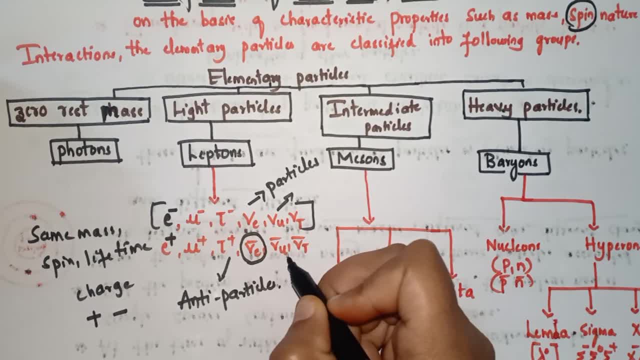 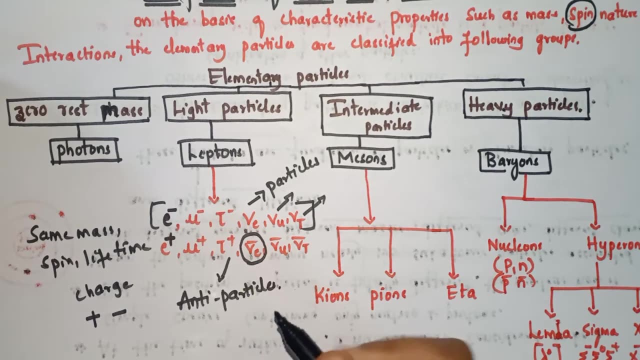 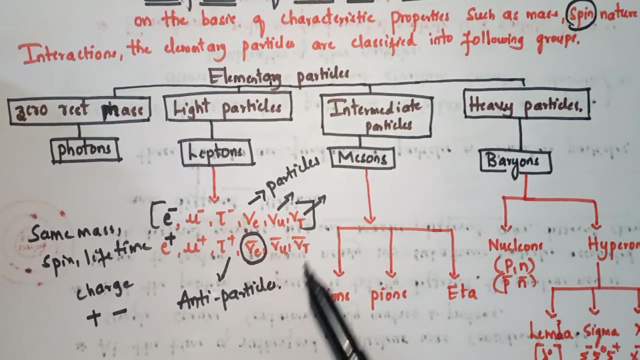 Mu antineutrino is an antiparticle and coming to this it is tau neutrino and antiparticle is tau antineutrino. See here the difference between the particles and antiparticle. that is, for the particles and antiparticles it is having same mass, spin and lifetime, but only difference is the charge. 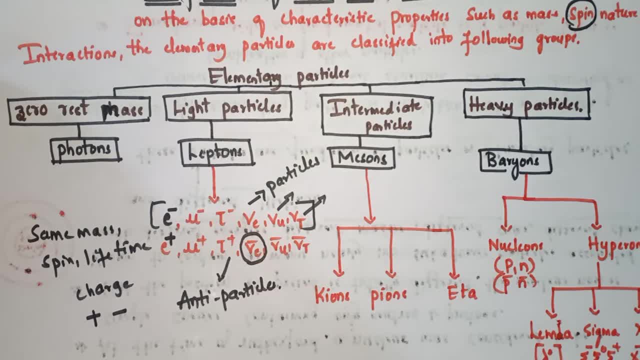 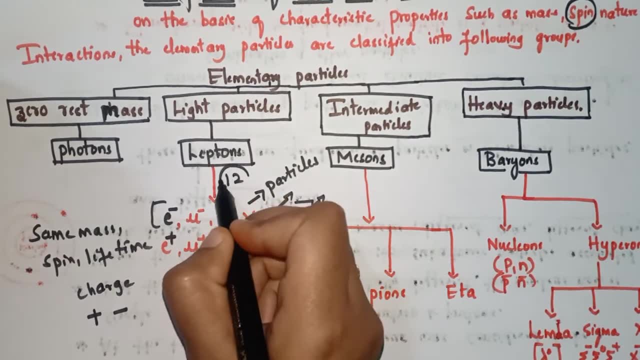 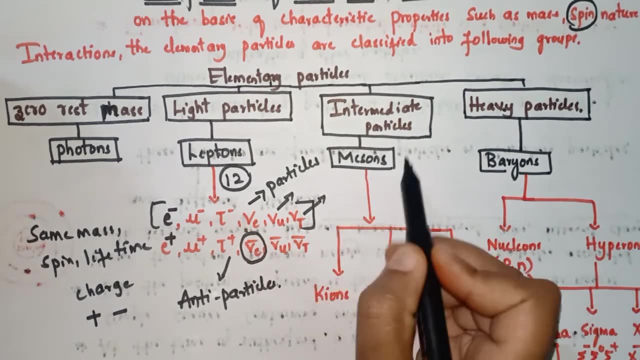 If it is having positive charge, the antiparticle will have the negative charge. This is about the classification of leptons, That is, they are classified into 12 particles. Now coming to the intermediate particles. Intermediate particles or mesons. 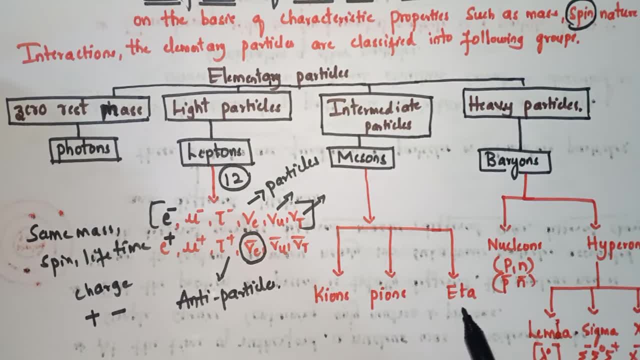 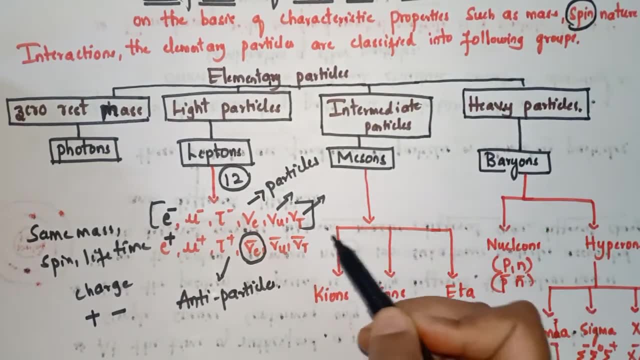 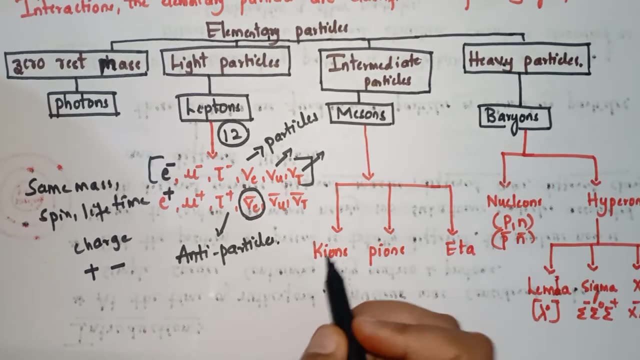 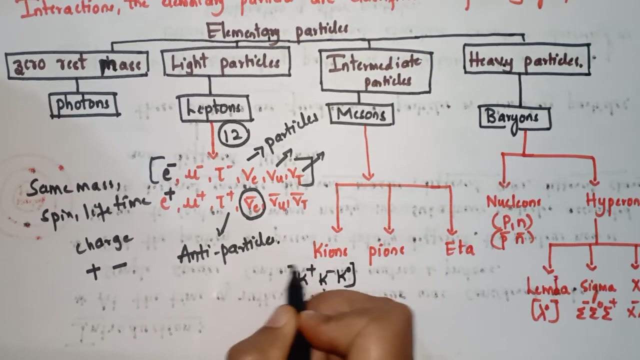 Mesons are classified into kaons, pions and eta. See here once again I will say you that is intermediate particles or mesons. they are classified into 3 types, that is kaons, pions and eta, eta. Now again, the k-ons are of three types, that is k plus, k minus and k naught. These are the 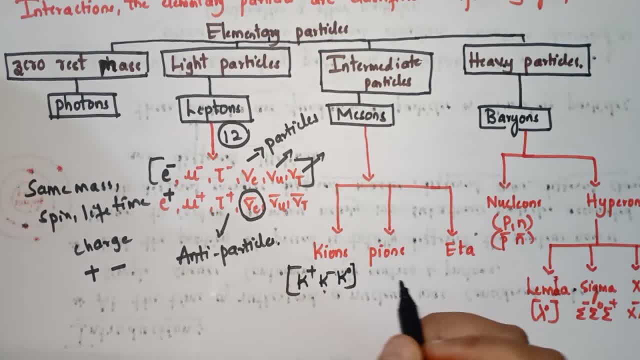 k-ons and for the pi-ons we are having three types, that is, pi minus, pi plus and pi naught. and for the eta we are having eta naught, only one. For the k-ons we are having k plus, k minus, k naught. For the pi-ons we are having pi minus, pi plus and pi naught. For the eta we are having 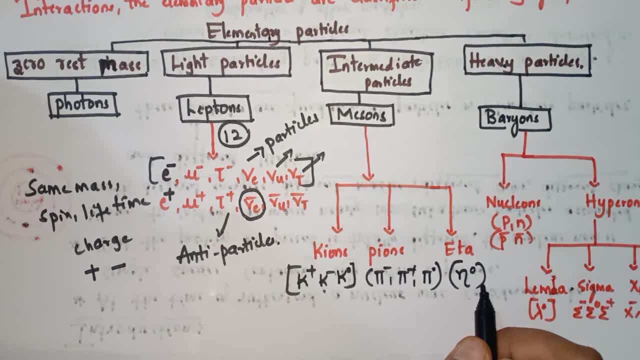 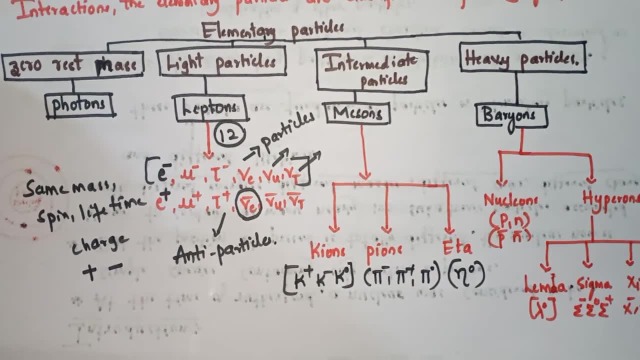 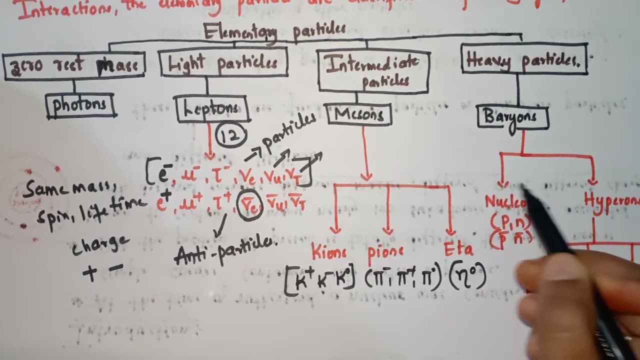 only one, that is eta naught. This is about the classification of mesons. Now coming to the heavy particles. Heavy particles or baryons. Baryons are classified into nucleons and hyperons. Nucleons are further classified into protons and neutrons. That is, the nuclear particle will include proton and neutron. For the proton, the anti-particle is anti-proton. For the neutron anti-particle is anti-neutron. Now coming to the hyperons. Hyperons are of four types. that is lambda sigma. 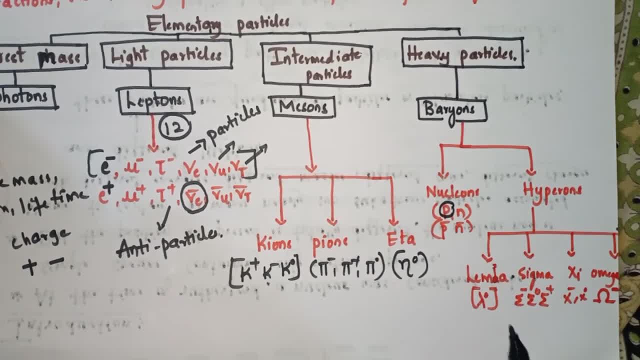 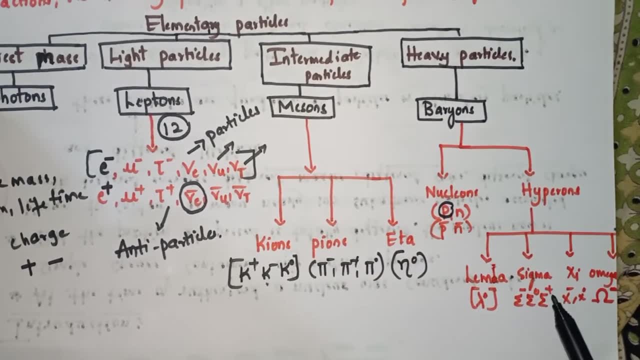 xi and omega. Here lambda is of only one, that is lambda naught. Sigma are of three types, that is sigma minus sigma naught and sigma minus Sigma naught. sigma plus and xi are of two types, that is xi minus xi naught and it is omega Omega. 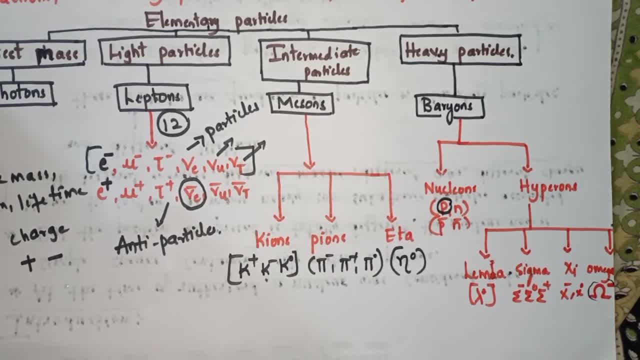 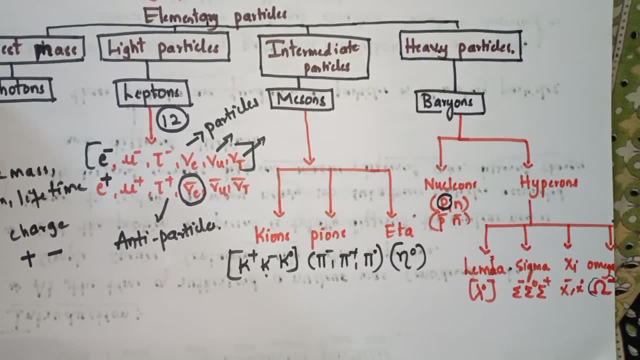 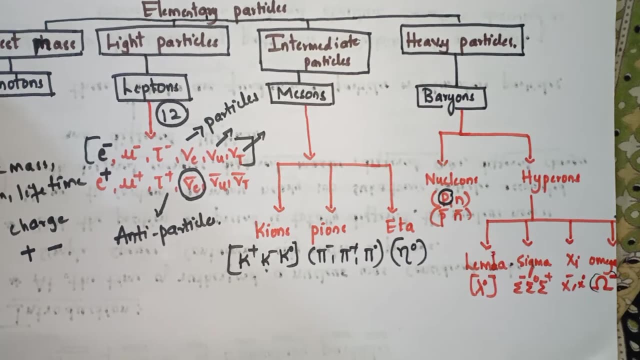 minus. This is the classification of hyperons. This classification is based on the mass spin and nature of interactions. And remember that particle and anti-particles have same mass spin, lifetime, but they are having opposite charge. And remember that for the electron. 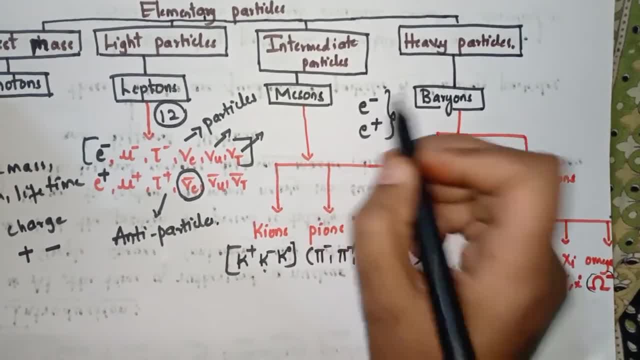 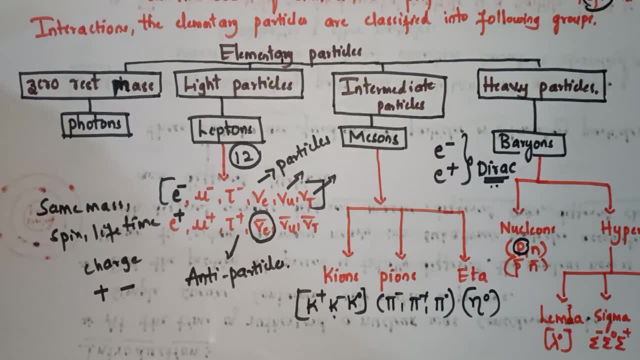 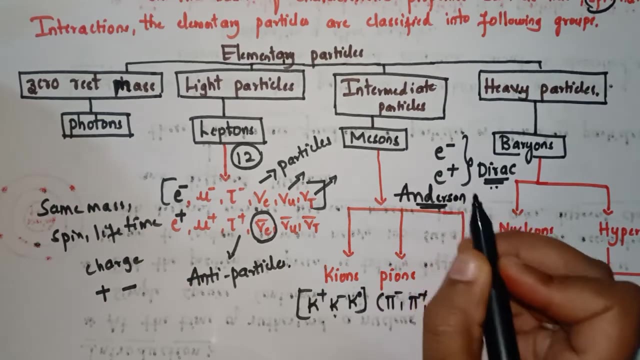 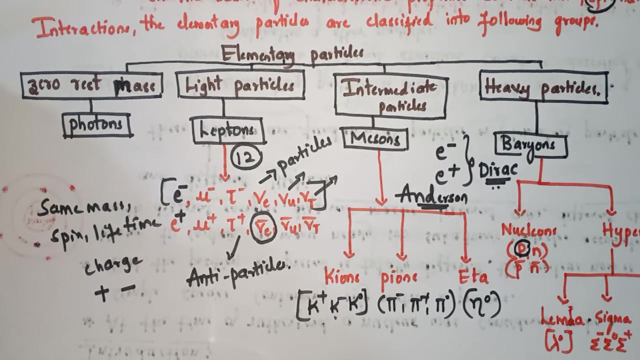 anti-particle is positron. This was predicted by Dirac. This is very, very important. This was discovered by Anderson, Anderson. Positron was discovered by Anderson, predicted by Dirac. Now I have to explain you the another important topic that is in these particles, which is having 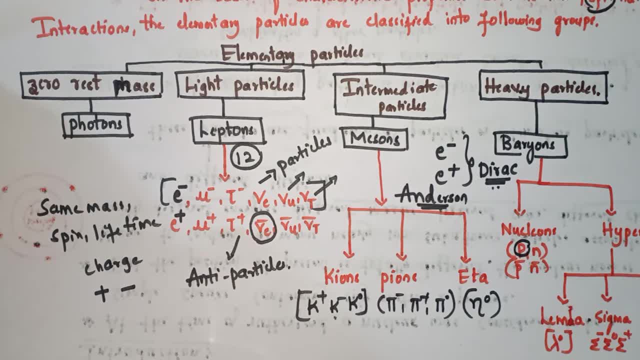 bosons and which is having fermions. Let's see that now To learn that we have to classify the elementary particles on the basis of spin. Then we will come to know that which are bosons and which are fermions, That is, which is having integral spin and which is having half. 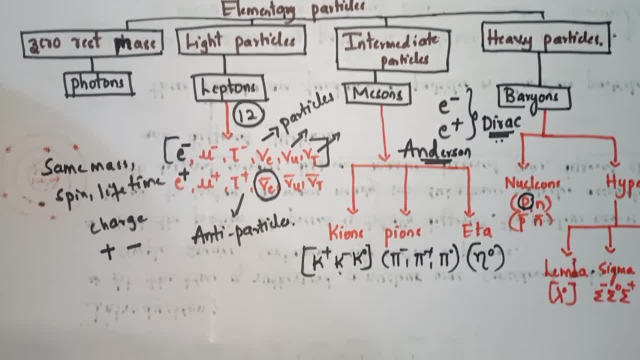 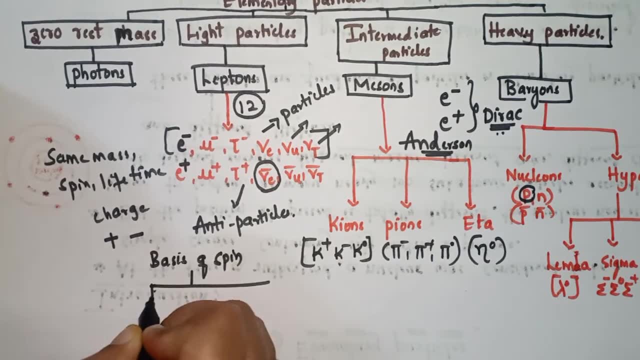 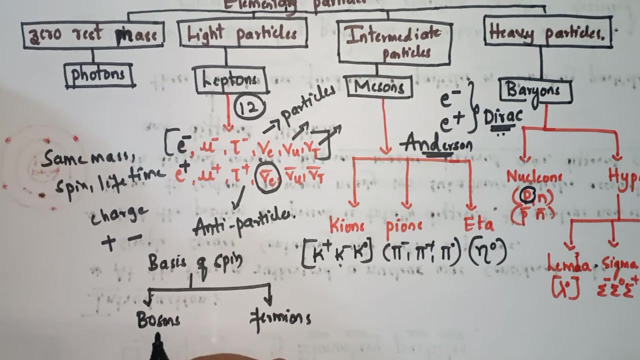 integral spin. See here on the basis of spin. on the basis of spin, listen it carefully. It is classified into two types, That is, bosons and fermions. Here bosons are having zero or integral spin. Zero or integral spin. 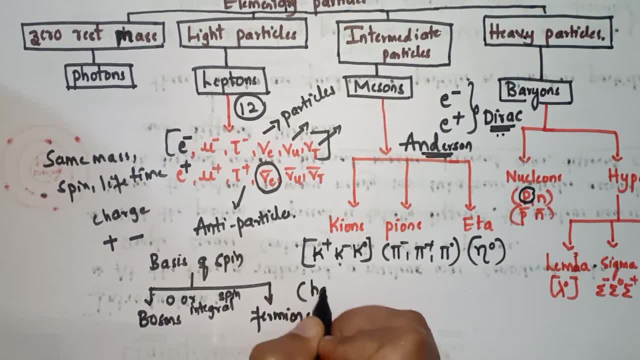 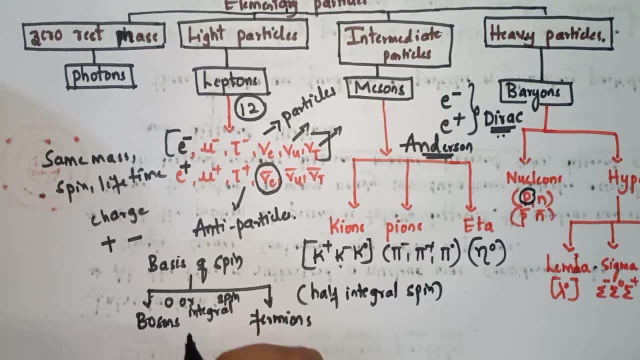 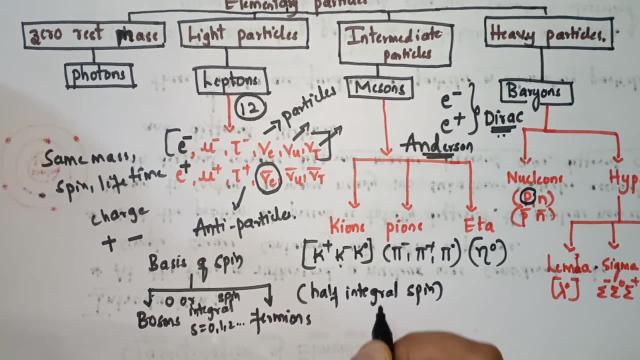 Whereas fermions are having half integral spin Here bosons are having, that is spin is equals to zero, one, two, etc. For the fermions the spin is of integral spin, That is s is equals to one by two, three by two, etc. 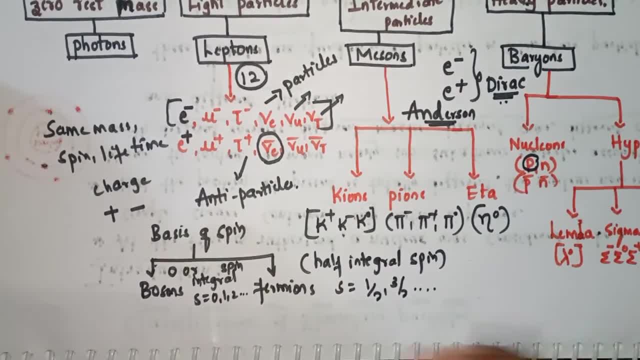 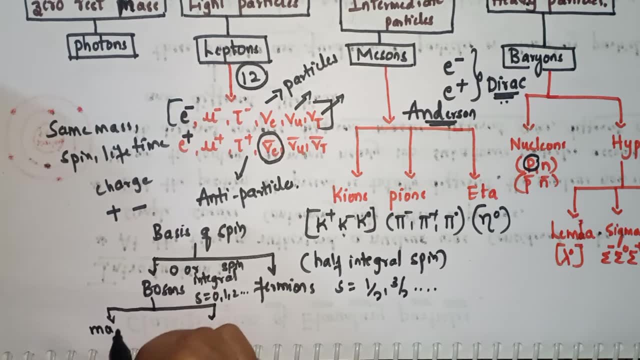 Now listen here carefully. Here bosons are again classified into two types, That is massless bosons, massless bosons, massless bosons and mesons- Here massless bosons. or photons and gravitons: Here these are of two types, That is photons. 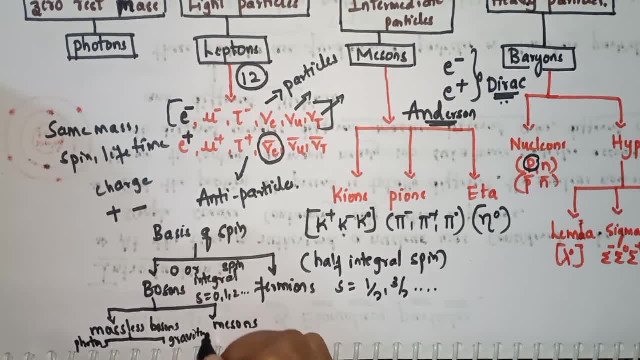 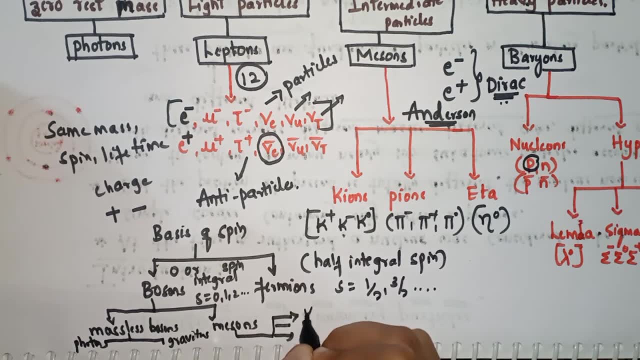 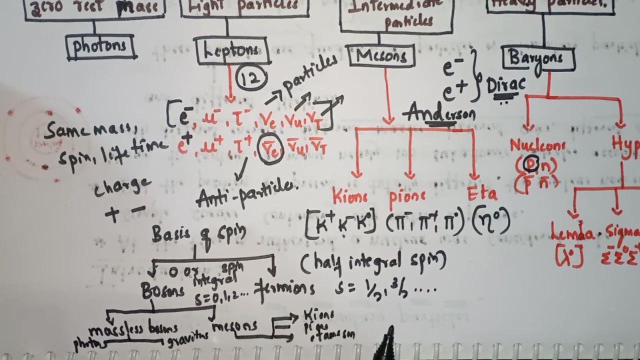 and gravitons. We know that mesons are three types, That is, k-ons, pi-ons and eatamasons. We already know that k-ons, k-music, k-k-4m-0 and ku-енты are classified into. See, the fermions are classified into Two types, that so-called leptons and baryons. 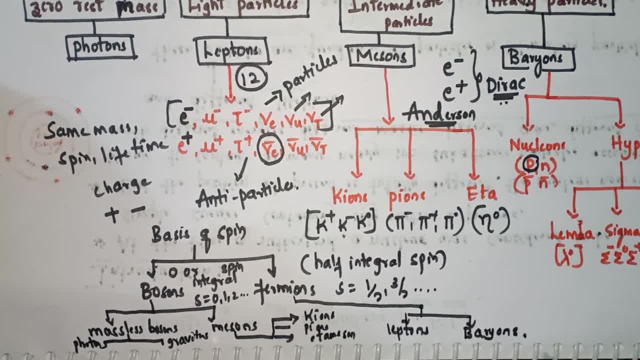 See, the fermions are classified into Leo and Leftons and baryons. That is Leptons and baryons, That is so, and so JE and Theph, Oracle, Leaptons and baryons. let me explain you once again on the basis of spin. here the elementary particles are classified. 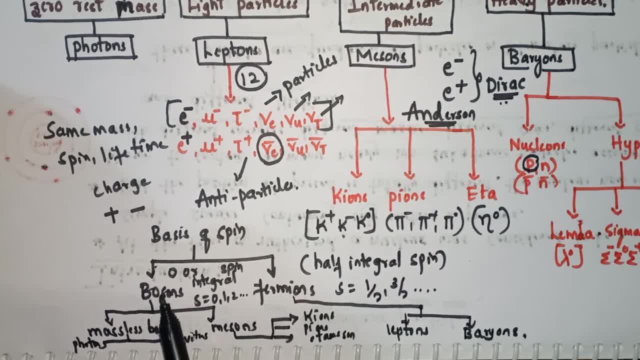 into bosons, or bosons and fermions. bosons are having zero or integral spin, that is sc. 0, 1, 2, 3, etc. whereas fermions are having of integral spin, that is sc is equals to 1 by 2, 3 by 2, etc. 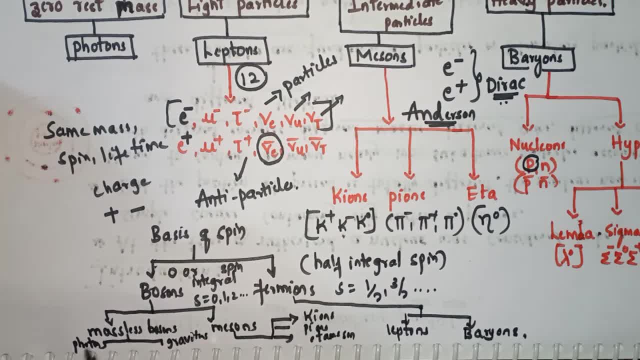 here. bosons are again classified into massless bosons and mesons. massless bosons are again classified into protons and gravitons, and we know that mesons are classified into kions, pions and eta mesons, whereas fermions are classified into leptons and baryons. see by this flow chart we 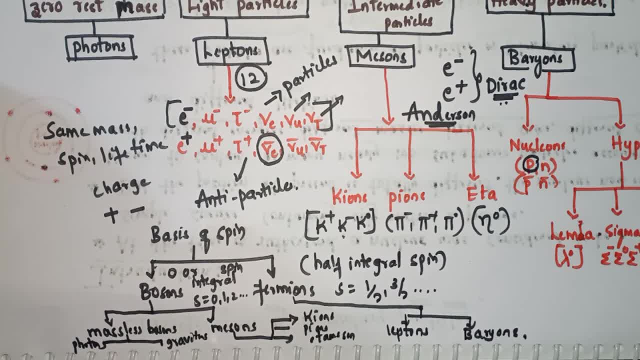 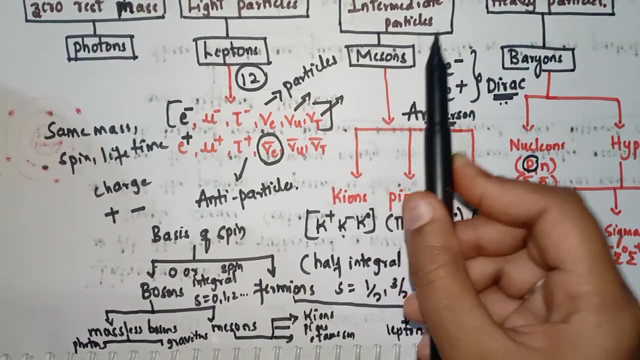 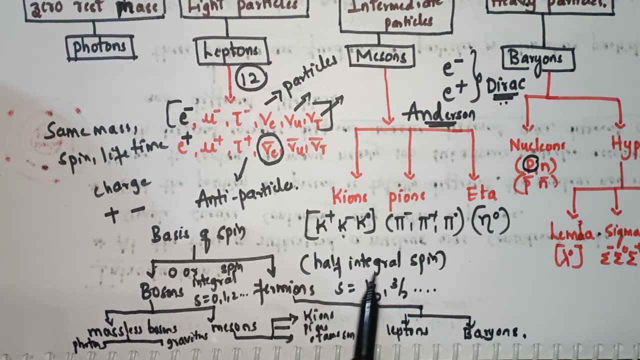 can understand that which is having zero or integral spin or which is having of integral spin. we can see that, say that here photons, gravitons and mesons, that is, photons and mesons are having bosons, that means they are having zero or integral spins, whereas leptons and baryons are having off integral spin. 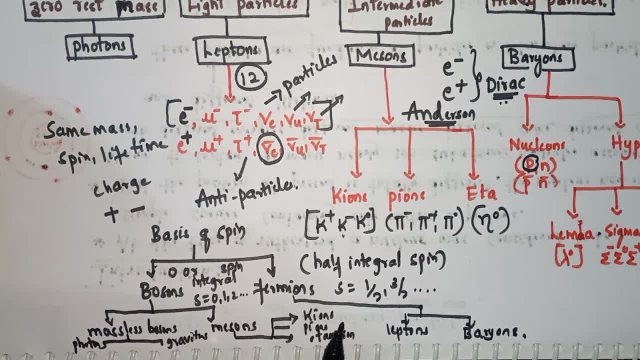 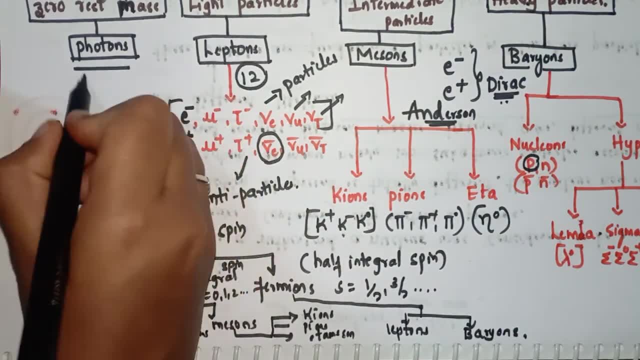 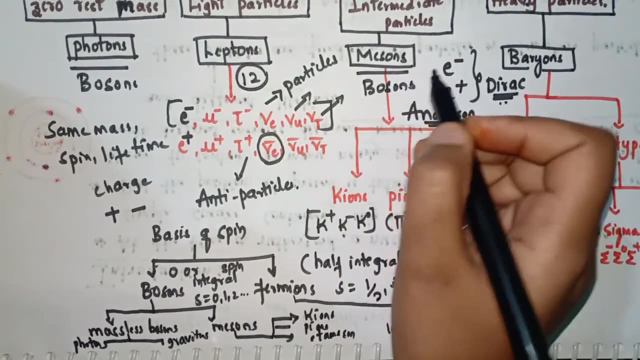 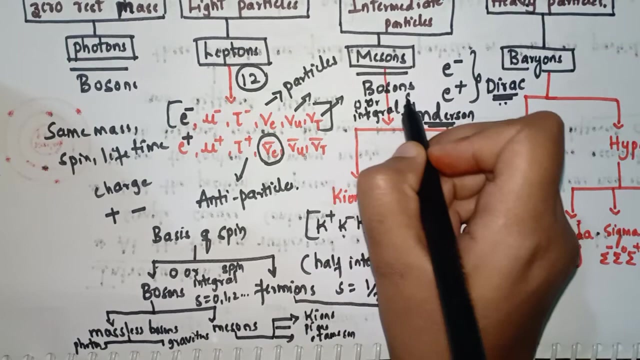 that is, they are having fermions. The purpose of this flow chart is to classify which are bosons and which are fermions. See, these photons are bosons and these mesons are bosons. that means they are having zero or integral spin. integral spin: this is also having zero or integral spin. 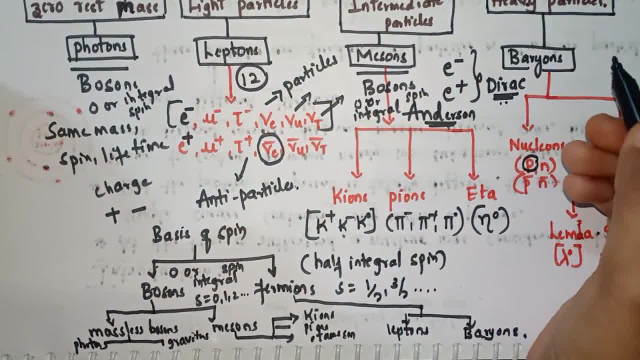 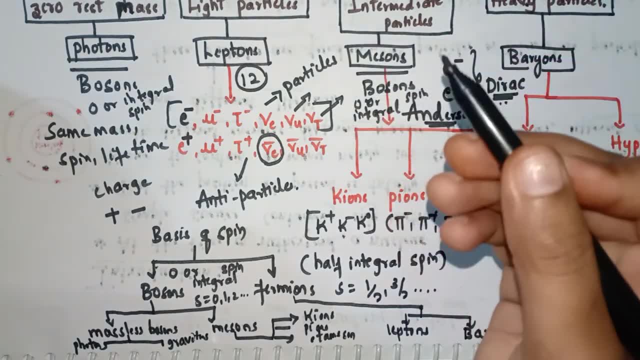 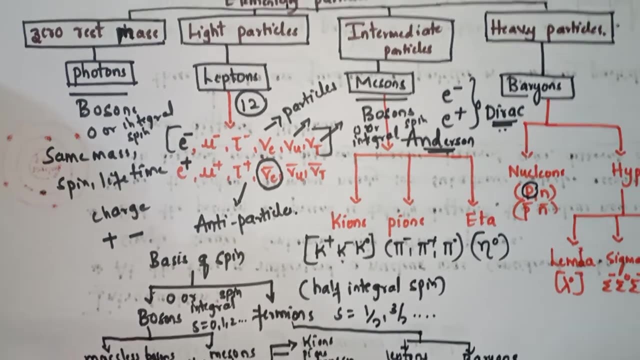 whereas leptons and baryons are fermions. leptons and baryons, or fermions, that means they are having off integral spin. that is 1 by 2, 3 by 2, like that. Now, if the question comes like this, for one max means that is what are photons? means you? 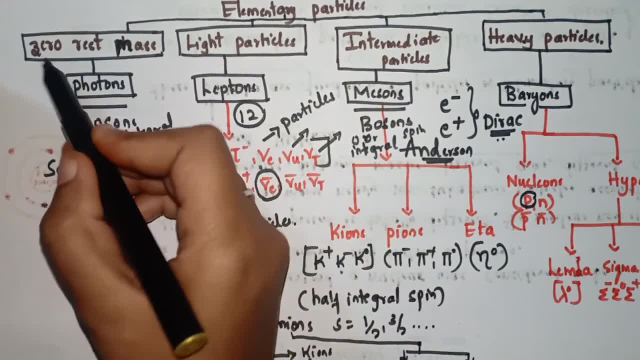 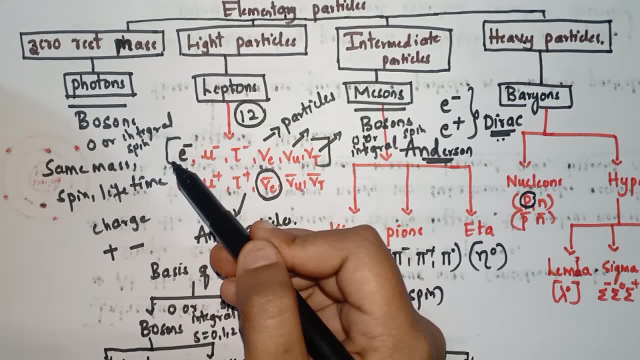 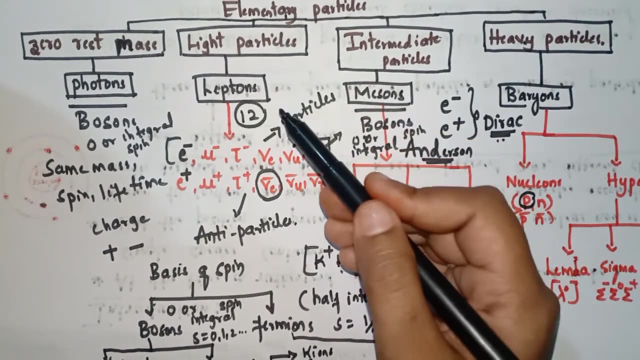 can directly say it is having zero rest mass and it is a boson. that means it is having zero or integral spin. If the question is about leptons means you can say that these are light particles which are fermions. that means they are having off integral spin. remember that. 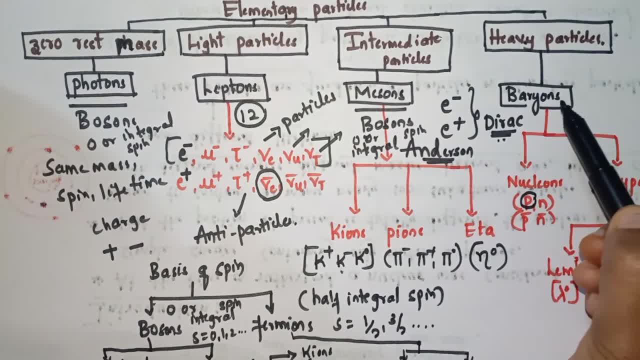 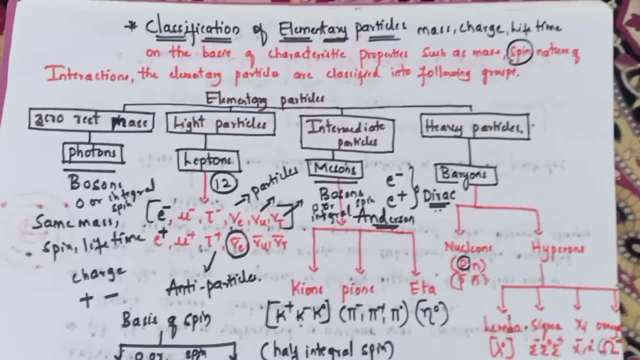 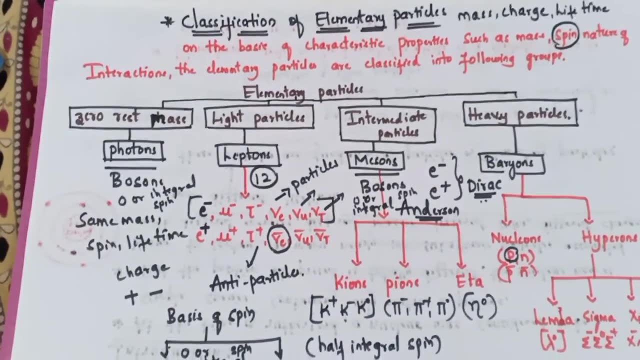 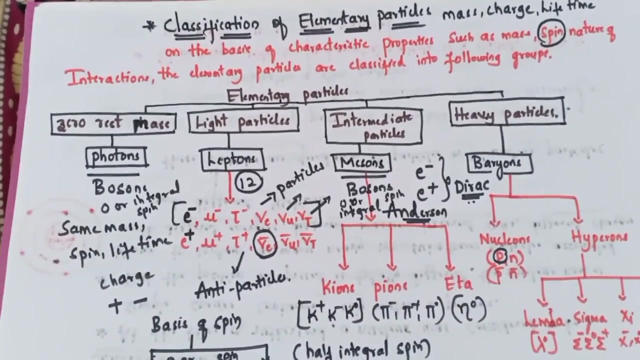 photons and mesons are bosons and leptons and baryons or fermions. i hope you all understood this classification very well. by this following explanation you should understand that the structure of nucleus is very, very complex. that is, in the nucleus not only proton and neutrons are present, but there are nearly 100 elementary particles. 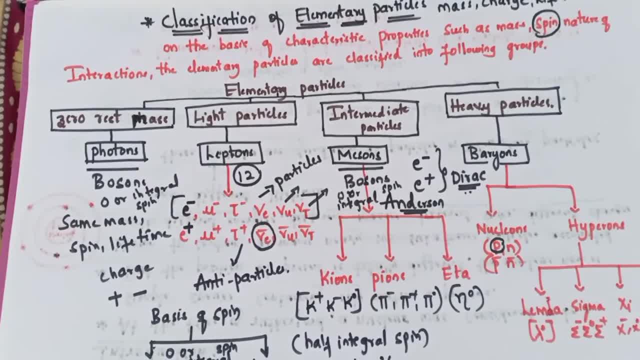 no theory has yet been developed to account for the origin of nearly 100 particles. thank you for watching. please subscribe to our channel.